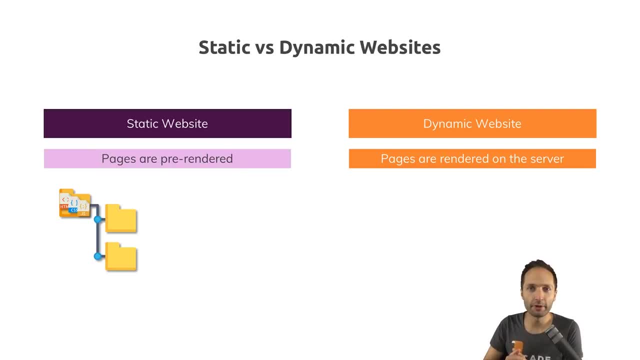 to visit our website, he will send a GET request to the server And he will get back the code that we saved or that we created right here. The same thing would be true if the user navigates to other pages on our website, for example. 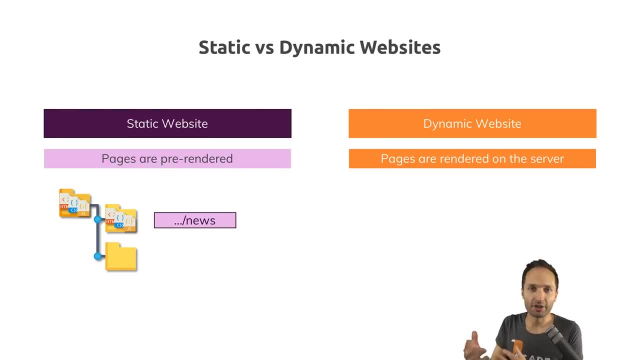 to a news page, Then we would also need another HTML file. That's important. So each new page of a static website needs an HTML file. It could optionally also include CSS or JavaScript, And the same thing would be true for another page like contact, for example. We would again. 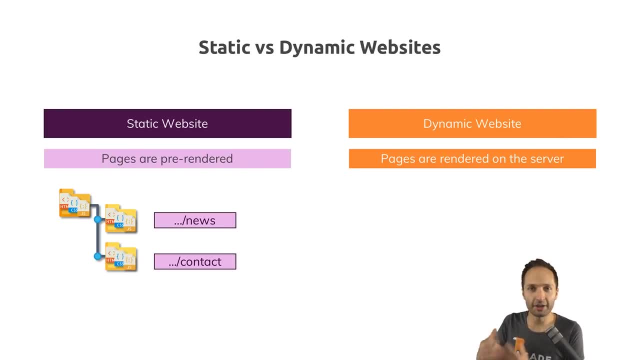 need an HTML file and, optionally, CSS and JavaScript. But the important thing is that we simply take the content and all that structure, save it on our website host, on our hosting provider. We will see that in a few seconds And that's it. The page is done and pre-rendered based on that code that we saved right here. 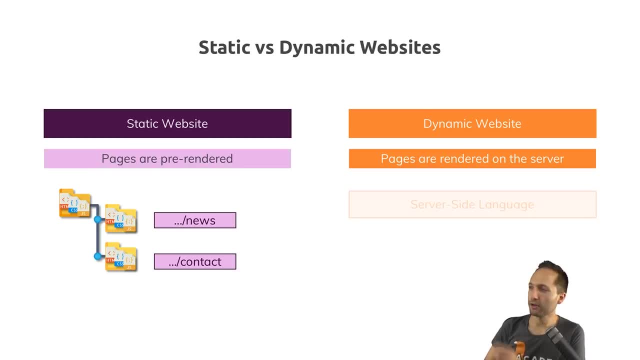 The dynamic website is a bit more complicated because a dynamic website requires a server-side language. This is something like PHP Node or Ruby or Ruby on Rails. Now I won't dive into the details behind dynamic websites now. As I said, it's a bit more complicated as 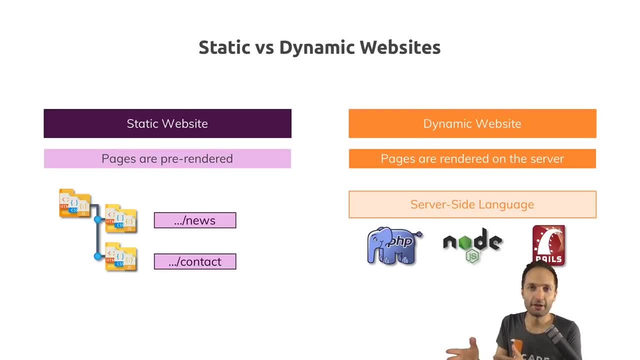 the content is not pre-rendered, So it's not just a thing like: take the files like we did it, save it on the server and that's it. It takes a bit more to host such a dynamic website, But in our case we have a static website, So the only thing we have to do- right? 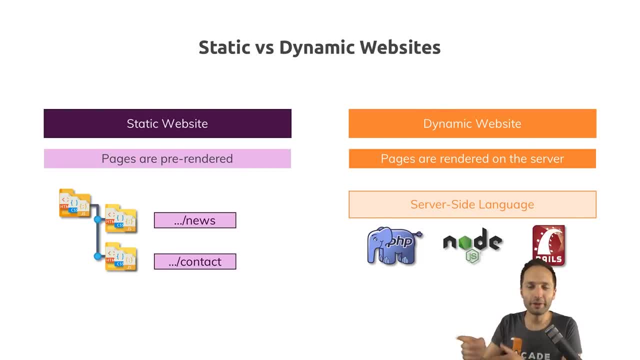 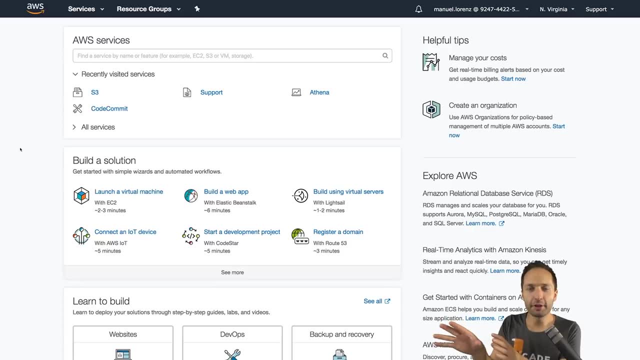 now is: We have to save our files on a server to make sure we can access it from the internet. How can we now host our static website? Well, in this video, I will use AWS to host our website right here. You can, of course, choose any hosting service provider of your choice. 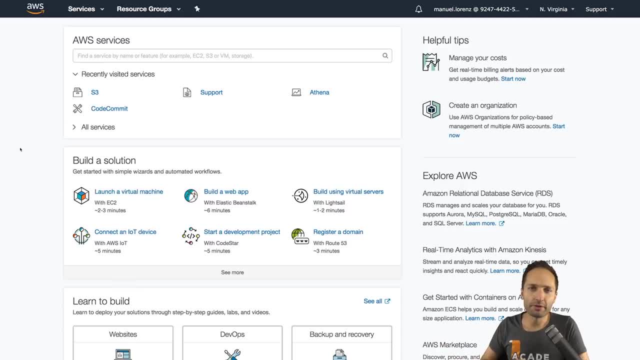 You could also use Firebase, for example, But, as I said, I will use AWS. In case you never heard about AWS before, we also got a complete getting started series here on the channel, So if you want to check this out, to understand what AWS is and how it works Now, as I said, 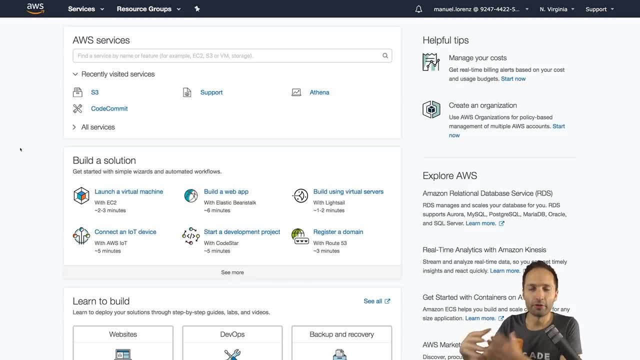 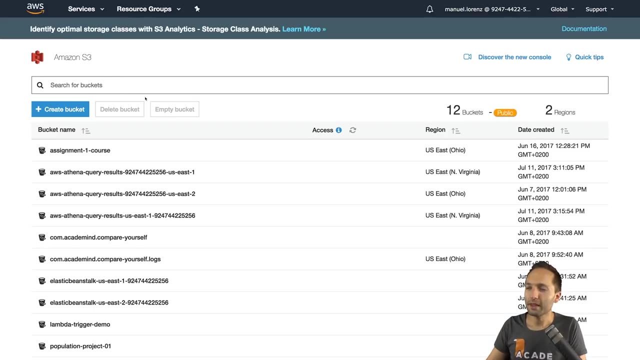 we want to simply store our website data on the server, And for that we need, well, a storage first. For AWS, we can use the S3, as it's written right here- the scalable cloud storage AWS offers. So let's click onto that And in S3, right here, we now have to create: 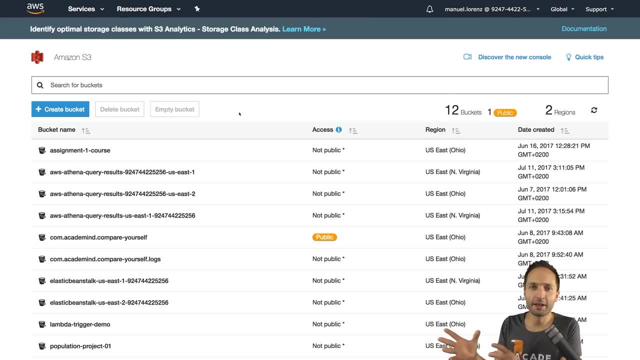 a so-called bucket. Now, this process, of course, takes a little bit of time, but it's very simple. It depends on the hosting provider you choose. I say that again because the steps outlined now are AWS specific, The important core step. that is always the same. 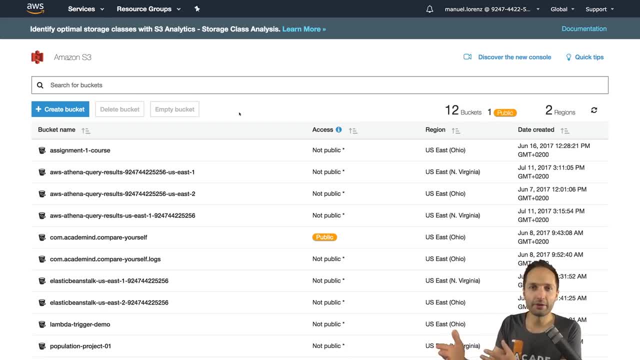 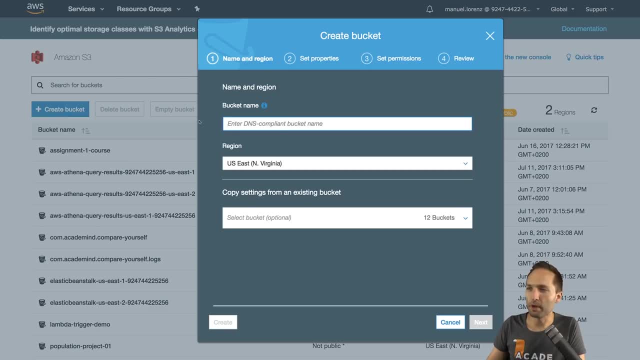 no matter which provider you're using, is that you have to save your data somewhere on a server in the internet. Now for AWS, we have to create a bucket. In that case, a bucket is something like a folder, And now we have to give this bucket a name. I will 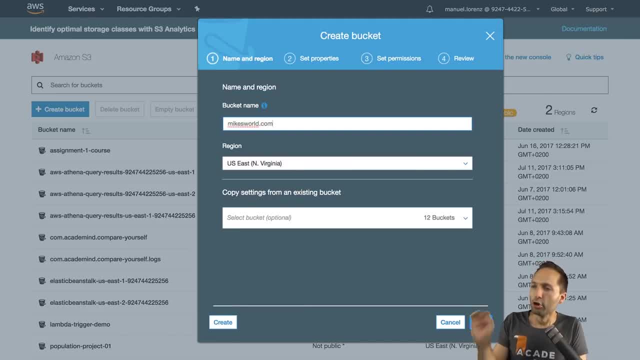 name it Mike's Worldcom. Normally you would name this according to the domain you registered, for example, in our case, academycom. I will show you quickly how you can register a domain at the end of the video. But for the purpose of our website right here, I will just use a dummy URL, which. 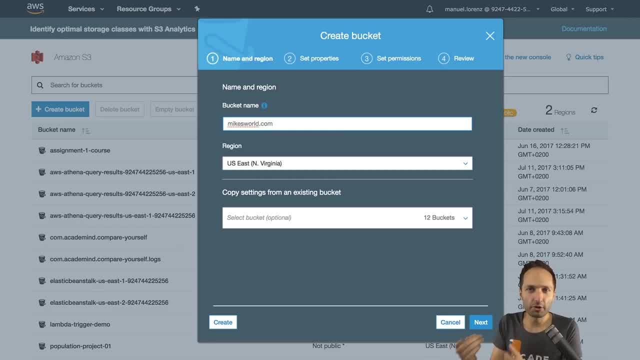 is generated automatically by AWS. It basically shows all the core features, But, as I said, normally you would register your own domain first and use this domain. So we have Mike's Worldcom right here. We can leave the settings the way they are, because the AWS standard 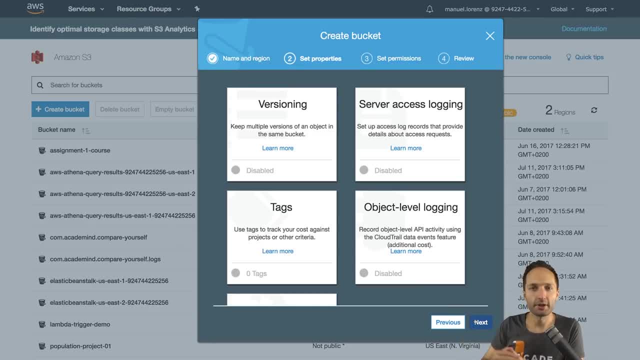 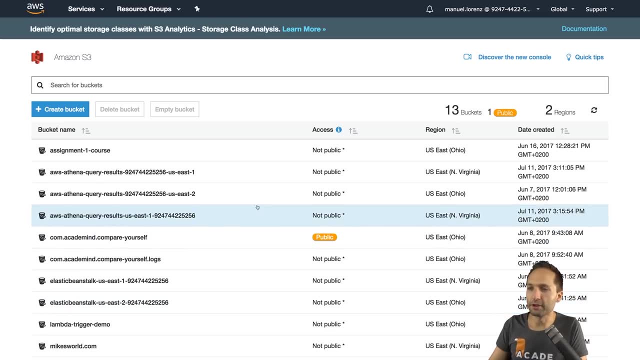 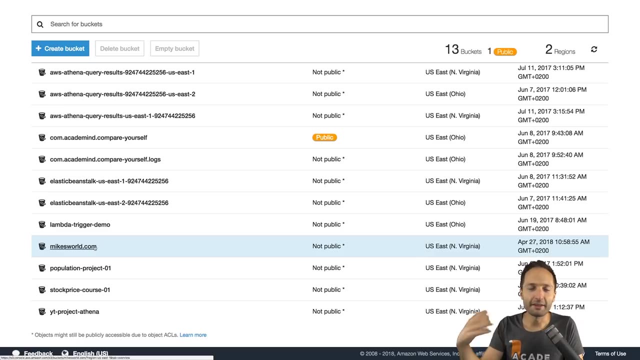 settings are always focused on to the highest security level. Therefore, this should be fine in most cases, So we can click Next and create bucket right here. With that, we got this bucket created And inside this bucket we now want to store the. 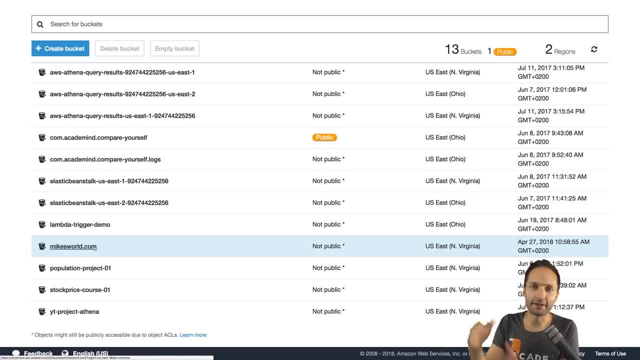 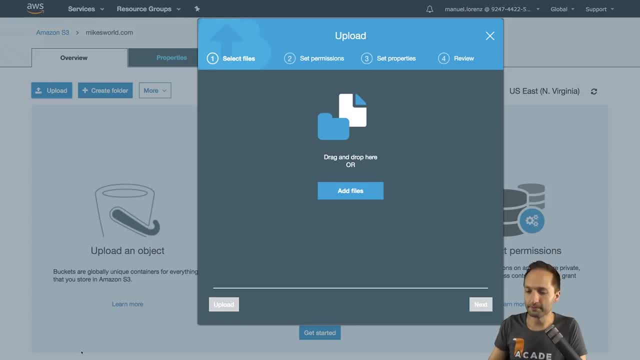 data we have for our website, So the HTML files, the CSS file and the JavaScript file. So let's click onto Mike's World now and select upload right here And now. I simply drag and drop the entire content So as you can see right here the files and the folder. 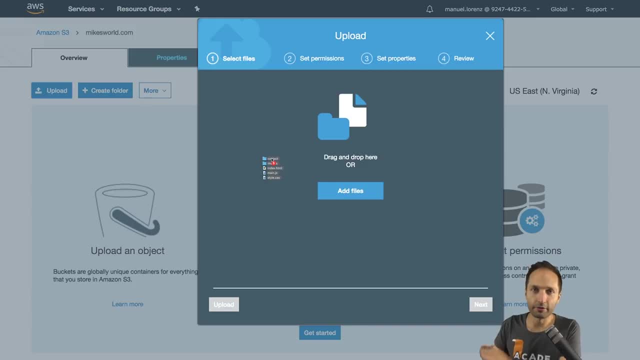 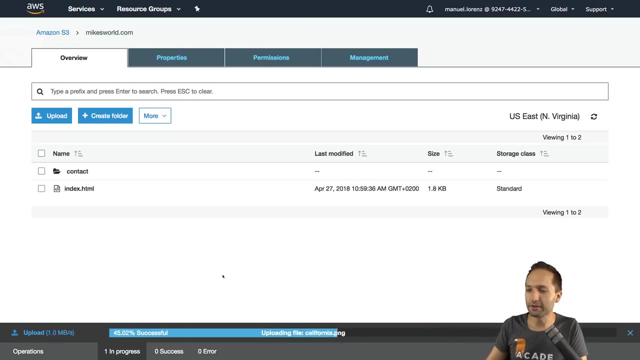 structure into this folder. You can find the code or link to the code attached to the video, of course, So let's drop it right here and press upload Now. it will take a few seconds And now we can see that we have all the different files stored right here in the bucket And 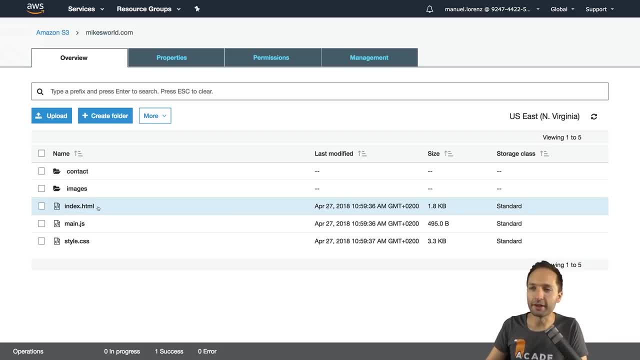 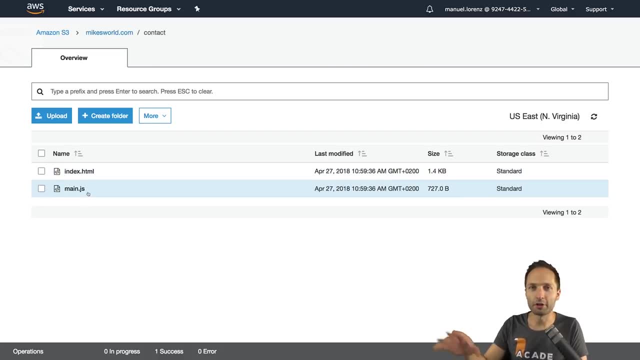 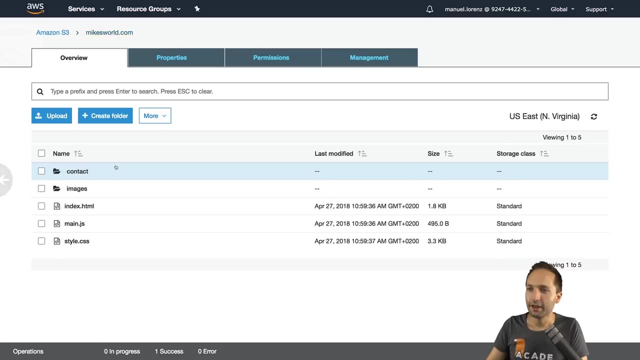 important. We have the landing page. So, with the index HTML file, the JavaScript file and the CSS file, And then we have the first sub page right here. This is our contact page And, as I said it before, on the slide we have a separate index HTML file for that page. 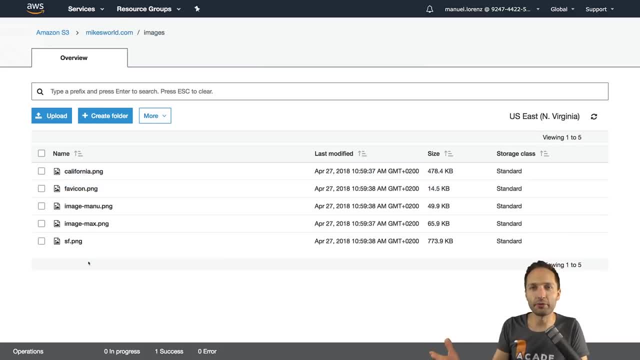 And if we go back and go to images, we can see that this is just the folder where our images are stored, So no HTML file required in this folder. However, that was the first step. We now simply save the files to a html file. 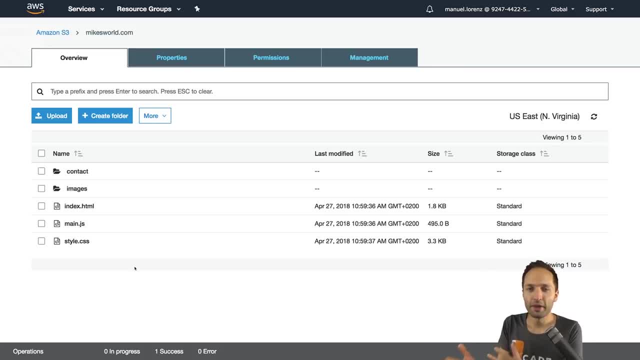 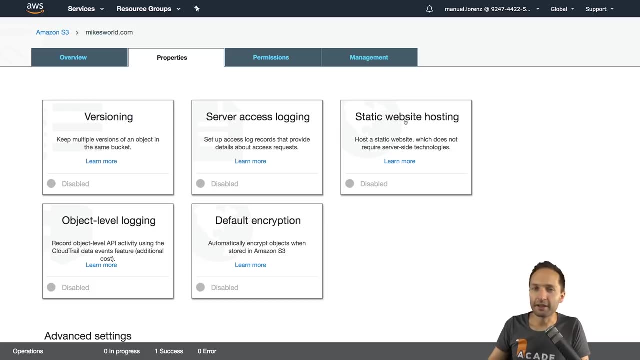 And now we can see that we have a static website hosting right here. This allows us to host a static website which does not require server side technologies. This would be a dynamic website, Also, something we had a quick look at in the beginning. 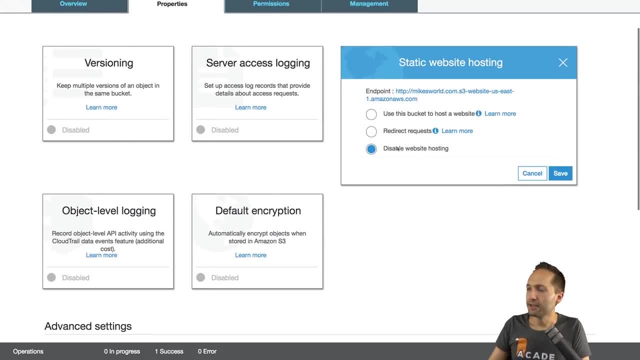 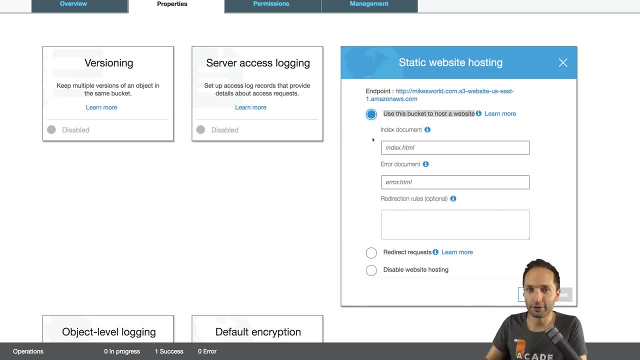 So let's press static website hosting. And now we have to select: use this bucket to host a website, because this bucket now contains the actual pre-rendered content of this website. And now we only have to do one thing and see another thing. The first thing we have to see is: is this endpoint right here? This is this dummy URL. 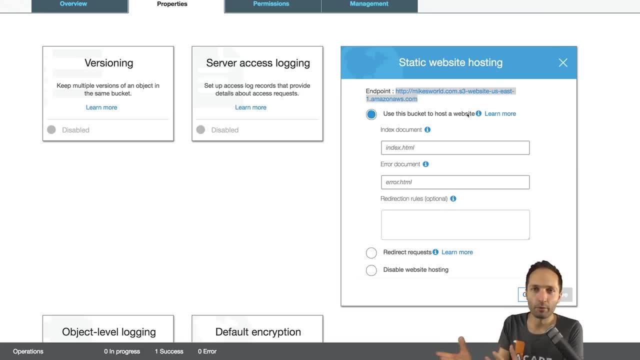 I just talked about. This is the end point right here. This is this dummy URL I just talked about. This is the URL we got right now from AWS because we didn't register a specific domain, As I said, for example, academycom. So let's copy this dummy URL, because this URL will allow us to 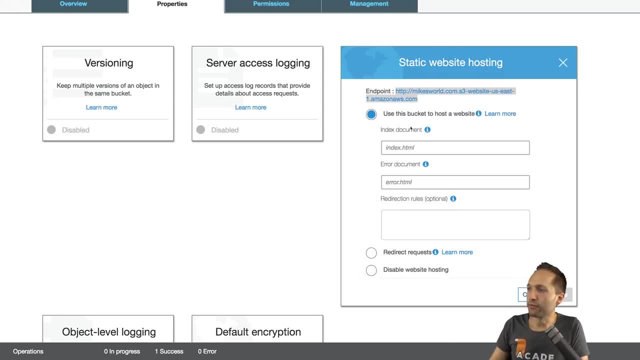 access our website from the internet then. So that was the first thing. The second thing is that we have to specify an index document, So basically a starting, a default document that should be loaded once we enter this endpoint, Endpoint, this domain up here, And this should indeed be the index HTML file, as we just saw. 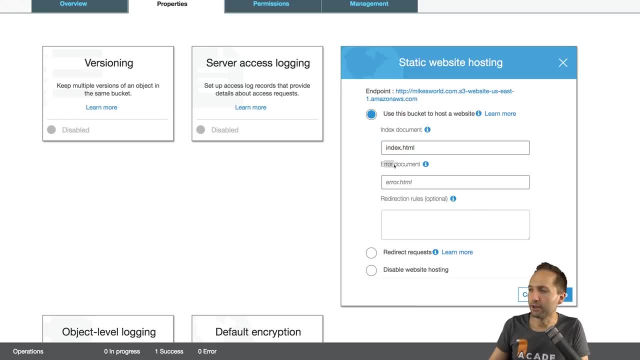 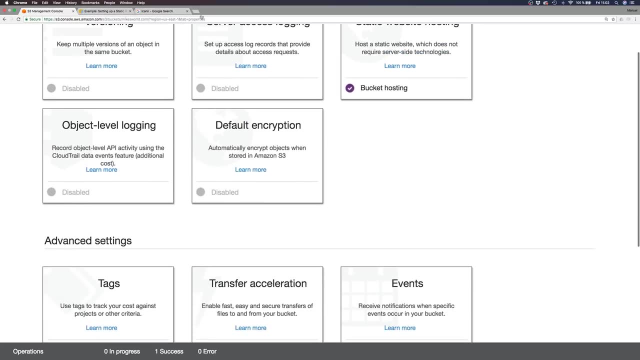 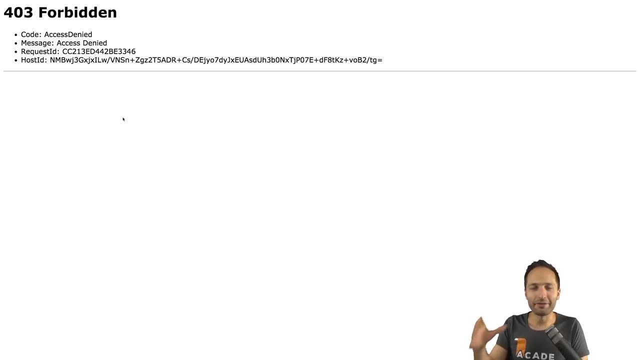 it. With that we are already done. We could specify an error document- not something we need right here- And if we now press save, we can go to a new tab right here and paste this URL and press enter. You can see that we don't have access to this website. This. 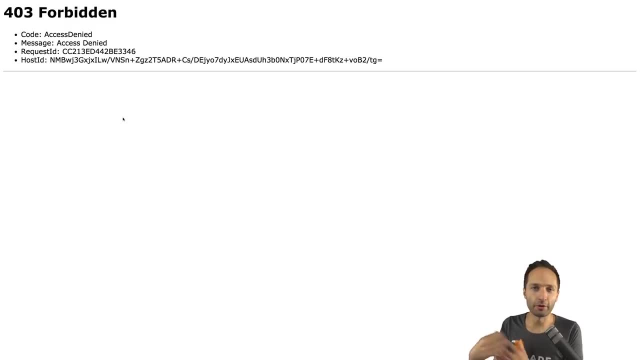 is also as free specific. Nevertheless, I wanted to show you this Because at the moment, we save the files in this cloud storage and we turn it into a server, But the problem is that, as I said in the beginning, we have the highest security settings. 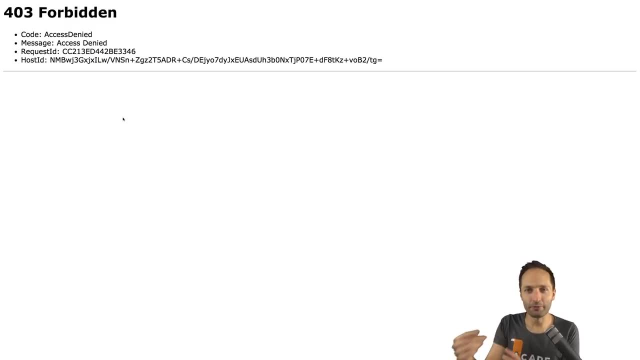 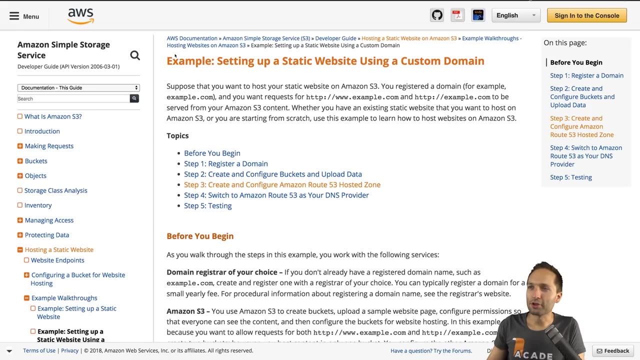 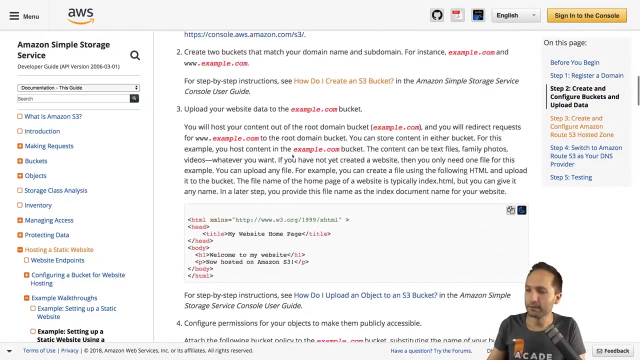 at the moment and therefore we are not allowed to access the information that is saved on this server. For that we need to go to the official documentation. A link can also be found in the video description, And if we now scroll down a bit right here, up to this: 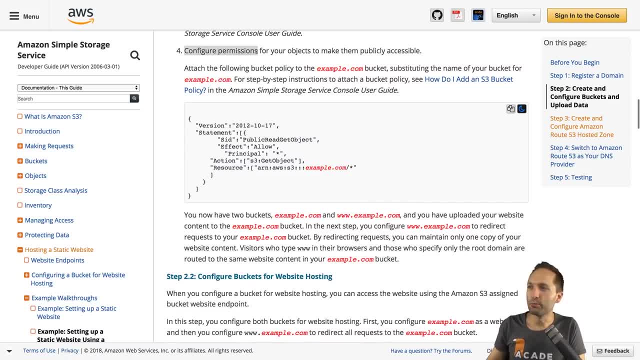 point. We can see that we can configure the permissions for the objects in our bucket to well as we can see it right here to make them publicly accessible. That's what we need. So let's simply copy this code right here by clicking onto this symbol right here. And if we now 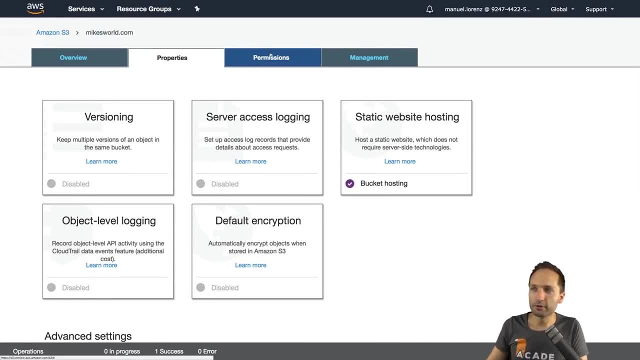 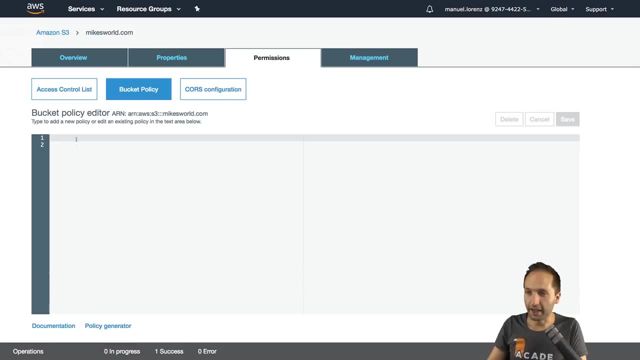 go back to our S3 management console and now go to permissions- right here- and now go to bucket policy- right there. Then we can paste this code. And now, important- we have to change examplecom with our mikesworldcom bucket name right here. This would normally 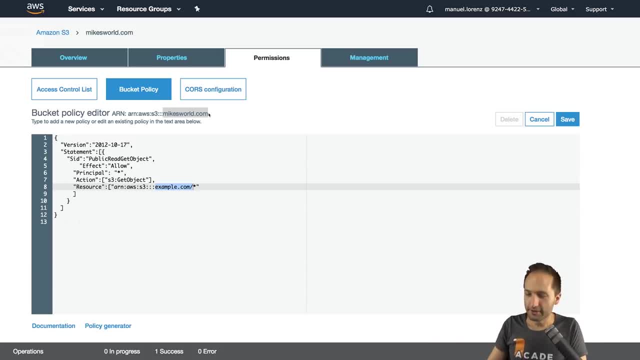 be the name of the domain you registered. So let's copy that and paste it right here like that. Don't forget to include the slash, otherwise this won't work, And if we now press save right here, you can see that this bucket. 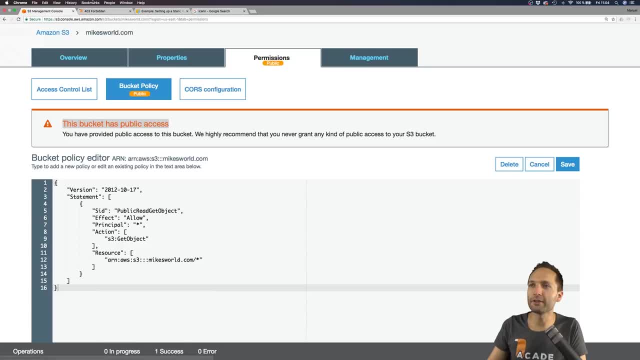 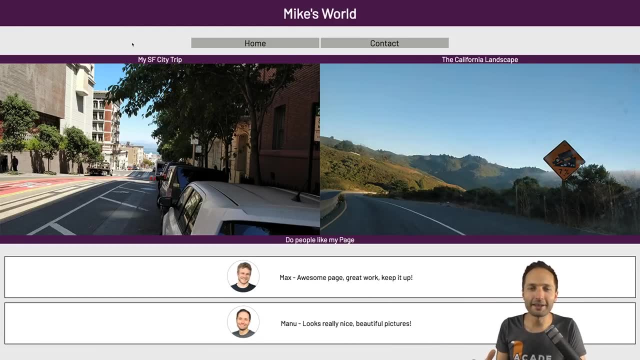 now has public access. So that's actually something that we want, And if we now go to back to our forbidden page right here and reload it, you can see that we can now access the content that we saved on the server and we can now display the website from the internet. so this means our 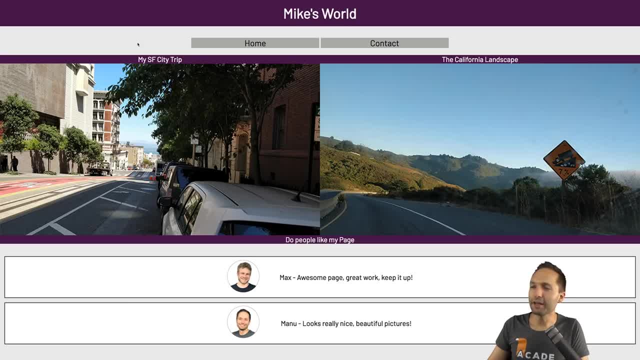 modal works perfectly. we can go to the contact page, so we can navigate around as we did it before, when we saved the file locally, but now we really have a server. this means the information is now well accessible from the internet, so everybody who has this url now can access our website. 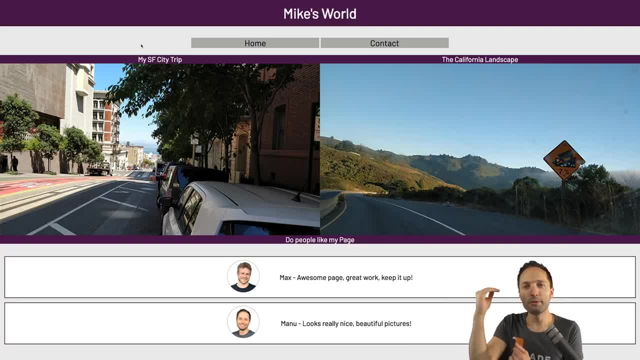 and additionally, if you remember back the beginning of the series, when we talked about the core concepts of how the web works, we can now finally send a get request to our server right here and, as a response, we get back the pre-rendered website as we can see it right here, and that's. 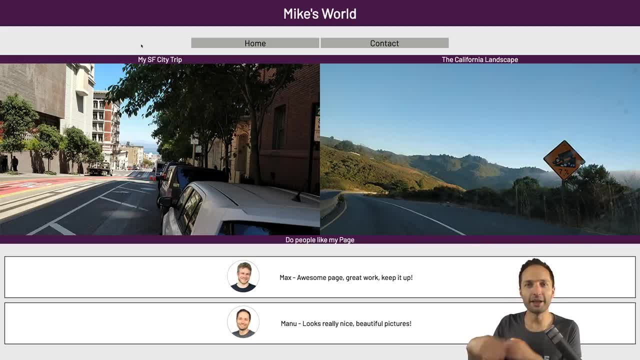 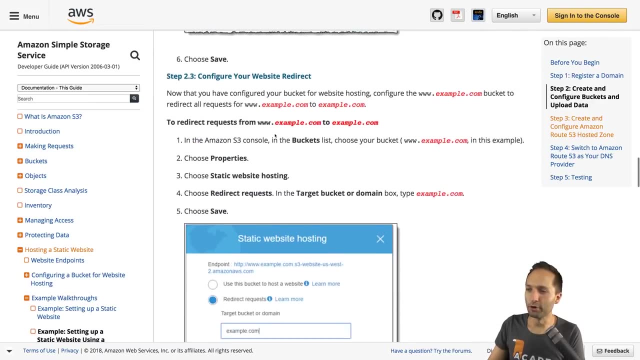 it actually. these are the actual core steps: to initialize the web, deploy your static website to the internet. there are some more important things i would like to add, though. the first thing is that if we go back to the official documentation and scroll down a bit more right here, these are all the steps that we did so far, but right here you can see that we 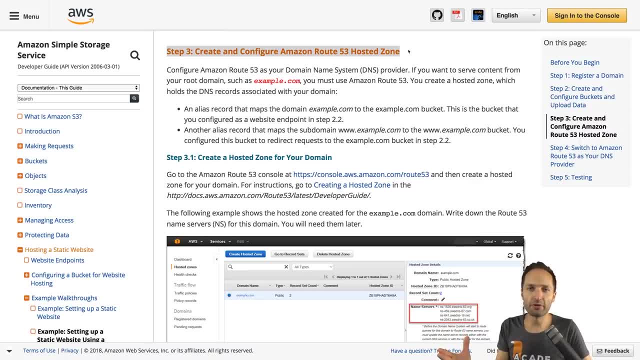 would now have to continue with step three if we want to host our website with aws and with our own domain. i will not dive into the details behind these steps right here in this video because, as you saw, if you just want to deploy your first website to the internet, not with an own domain but with a dummy domain, the steps we did. 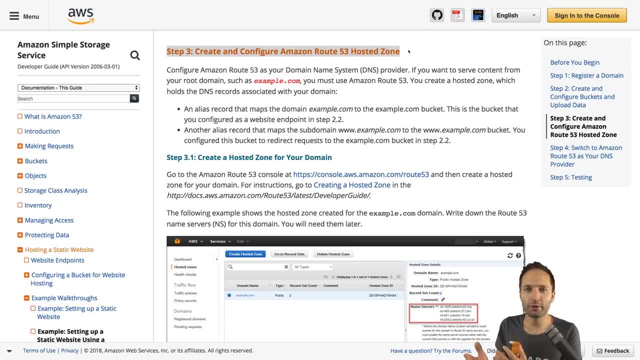 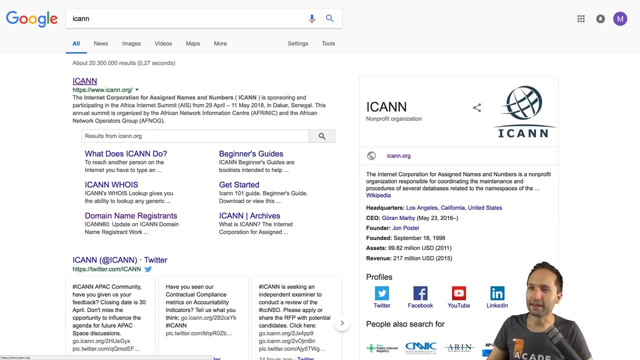 so far are everything you need now. in case you want to have your own domain, as i said, you have to continue with step three now and you also need an own domain, of course, for that you can simply google right here, for i can- and if you click onto this link, then 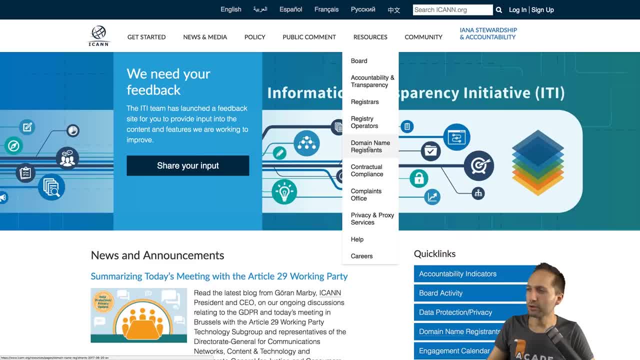 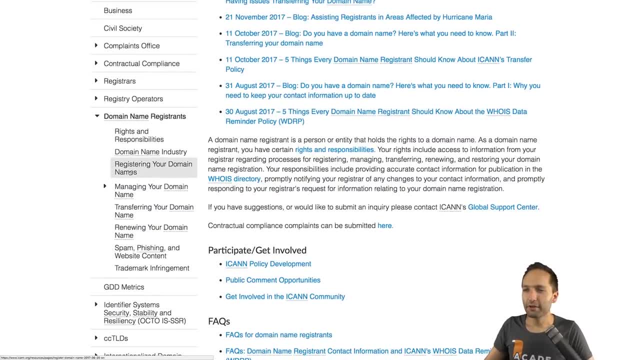 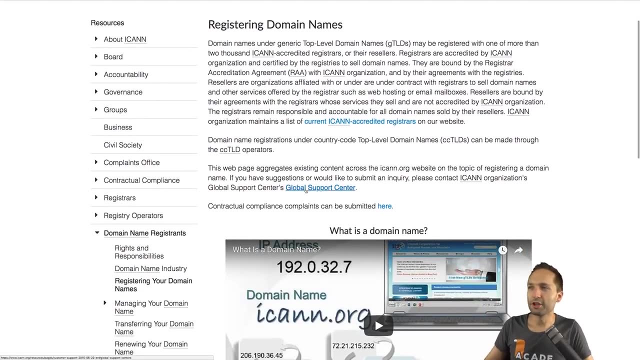 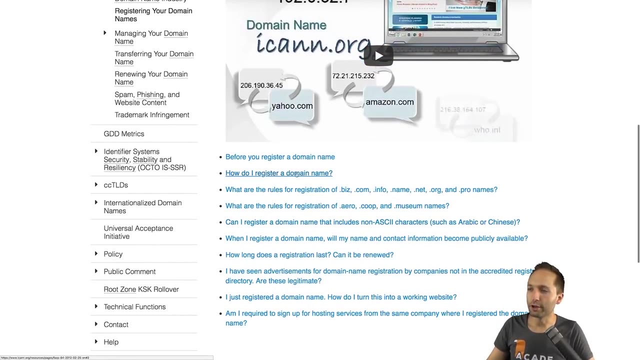 then go to resources and now go to domain name registrants right here. then you can scroll down a bit and then select right here registering your domain names. if you click onto this link, then you can well find some information about domain names, how it works, and you can also find a video right here, but you can also find the link right here: how do i register? 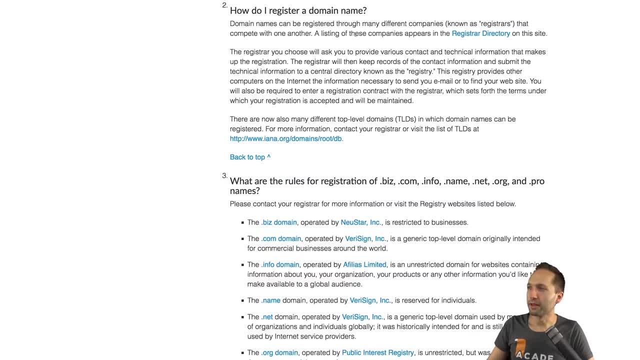 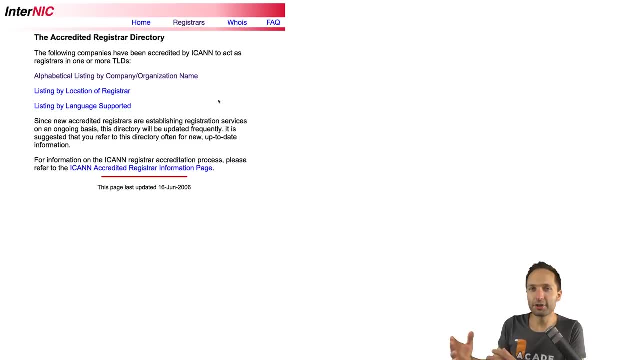 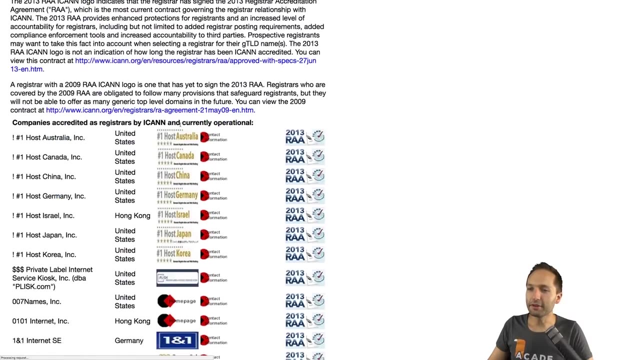 a domain name. if you click onto this link and then right here in this part onto the register directory, then you can find a list of the pages that allow you to register a domain. so if you click onto the first link- alphabetical listing, for example- then you can. 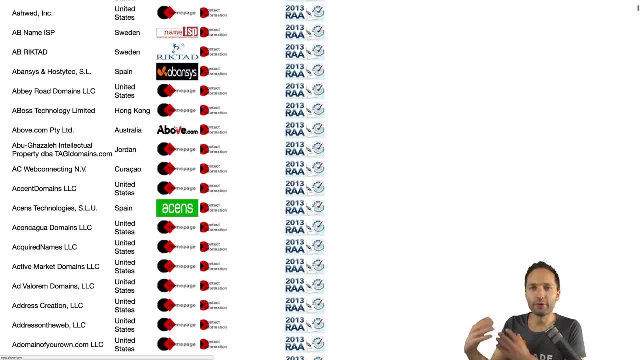 find the link of a lot of different providers which allow you to register a domain, so that's also something you might have want to look at if you want to register your own domain and by that set up your own home page. but generally, that's it now. this was the last video. 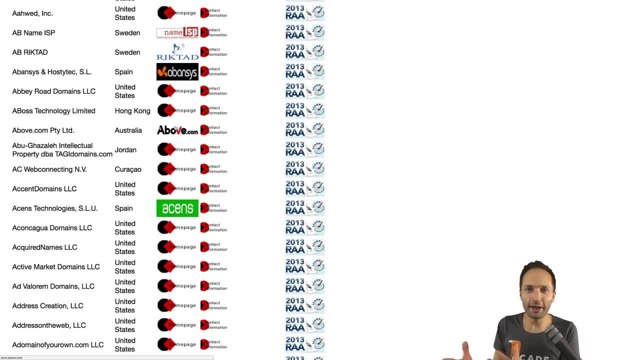 of this beginner's guide and, as i said in the beginning, i think we had a look at a lot of different core concepts of html, css and javascript, and also of how the web in general works. so i hope you enjoyed this series and i hope you found some interesting information that you can also use in. 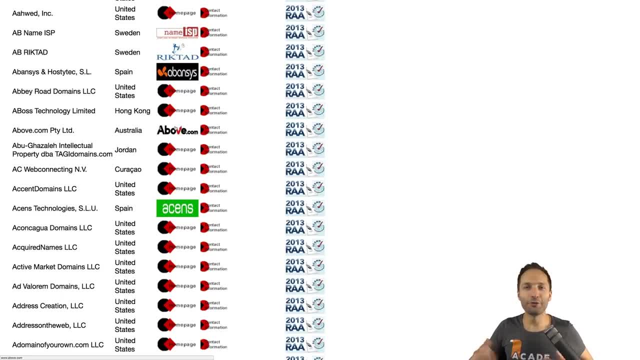 your own projects. so the only thing i can say right now is: thanks a lot for watching this series and i hope to see you in one of the next videos. bye you. 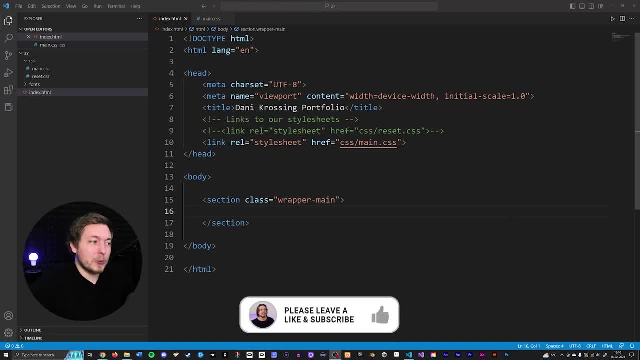 Today, you're going to learn how to create a form inside your website, And creating a form is something that is very useful, but probably not right now. The reason I say that is because forms are usually used when it comes to submitting data from the user. So let's say you have a. 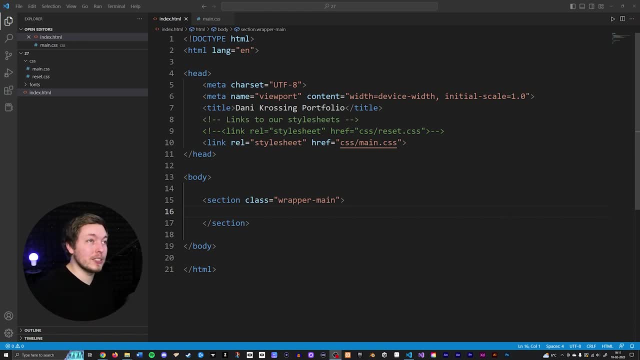 website. you have a contact form or you might have a login system or a signup form. You know we can go in and you can type in your name and your username, your email, and then you can submit it. This is usually what we use forms for. So in a lot of cases, when it comes to actually 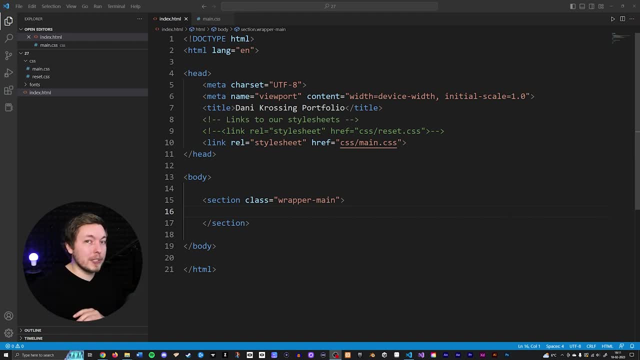 using the data from the user. you do need to have another language, like, for example, JavaScript or PHP or Python or something that can actually do something with this data, And at this point, a lot of people are probably considering clicking away from this video. 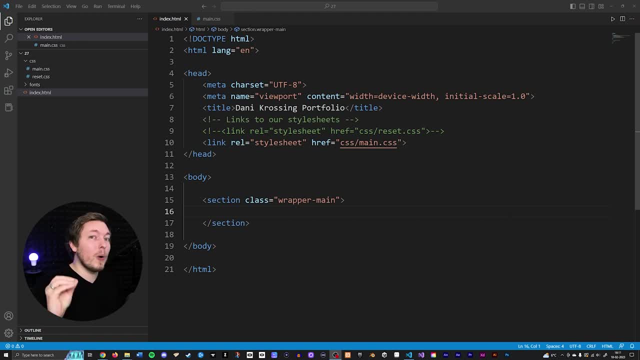 And I just want to mention that it is important that you know how to create forms before you get to that point where you have to start learning PHP or JavaScript or Python Or whatever. So once you get to the day where you actually learn how to do something with this,